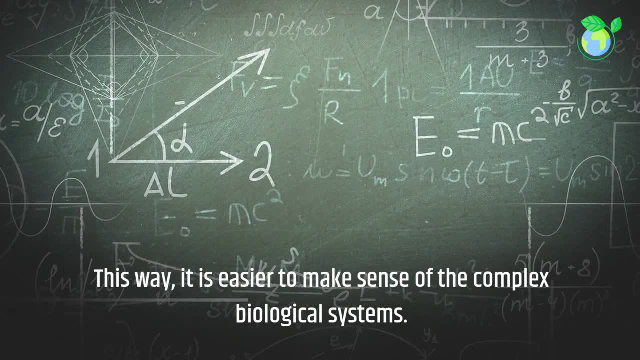 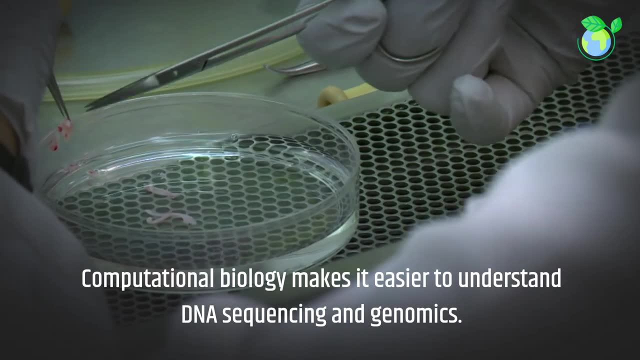 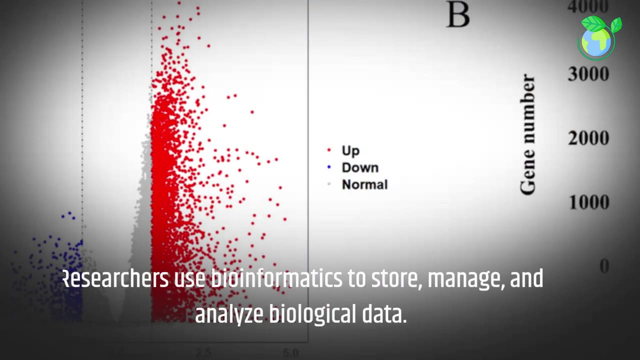 This way, it is easier to make sense of the complex biological systems. Computational biology makes it easier to understand DNA sequencing and genomics. It also helps researchers create new organisms and biological systems. Researchers use bioinformatics to store, manage and analyze biological data. 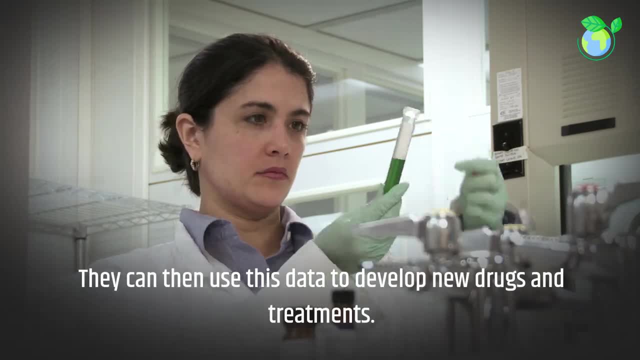 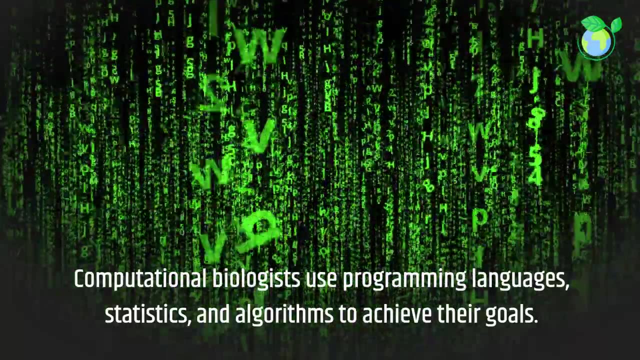 They can then use this data to develop new drugs and treatments. Computational biologists use programming languages, statistics and algorithms to achieve their goals. This results in a more efficient and efficient biotechnology. This results in a more efficient analysis, interpretation and modeling of biological systems. 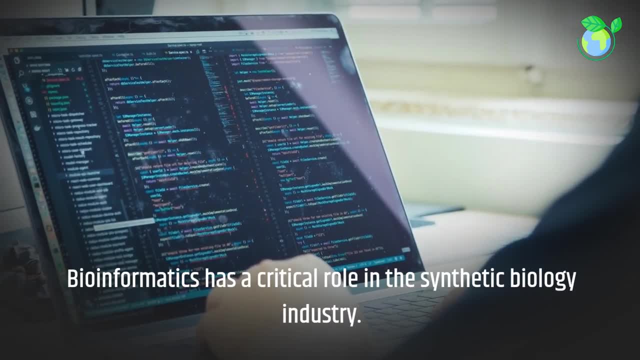 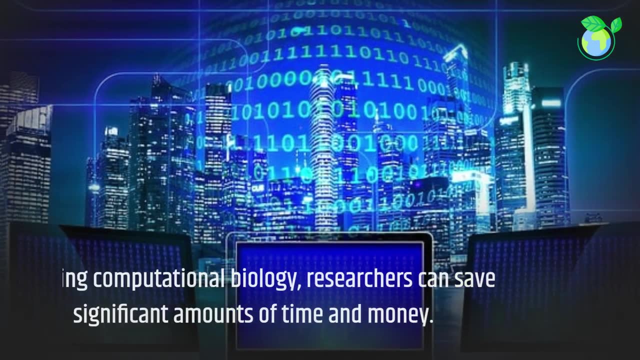 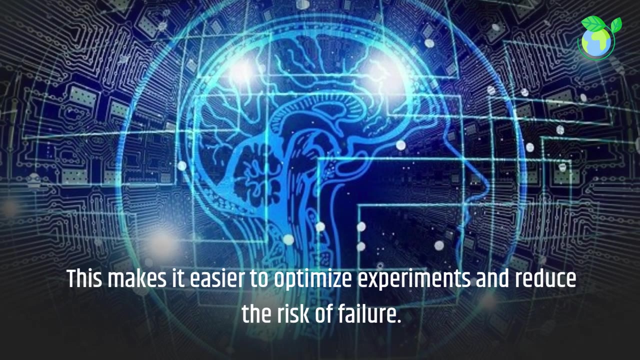 Bioinformatics has a critical role in the synthetic biology industry. These tools help researchers design and model synthetic biological systems. By using computational biology, researchers can save significant amounts of time and money. This makes it easier to optimize experiments and reduce the risk of failure. 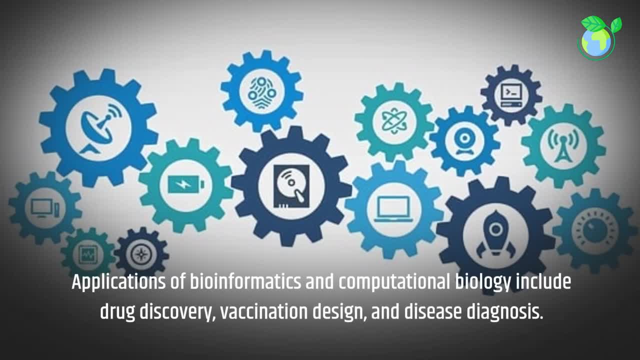 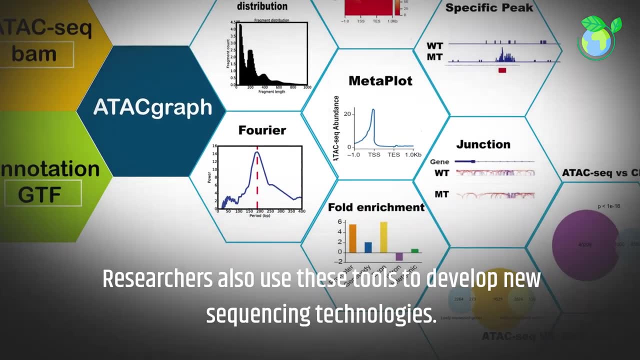 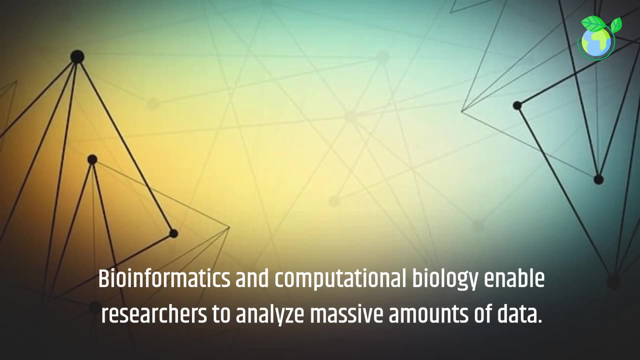 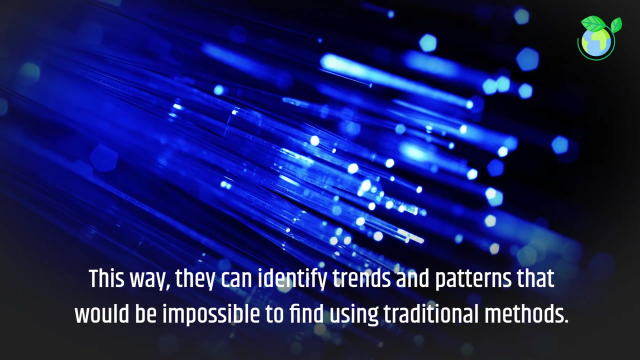 Applications of bioinformatics and computational biology include drug discovery, vaccination design and disease diagnosis. Researchers also use these tools to develop new sequencing technologies. Bioinformatics and computational biology enable researchers to analyze massive amounts of data. This way, they can identify trends and patterns that would be impossible to find using traditional methods. 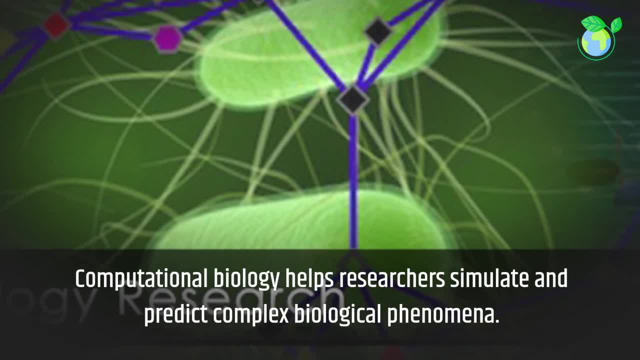 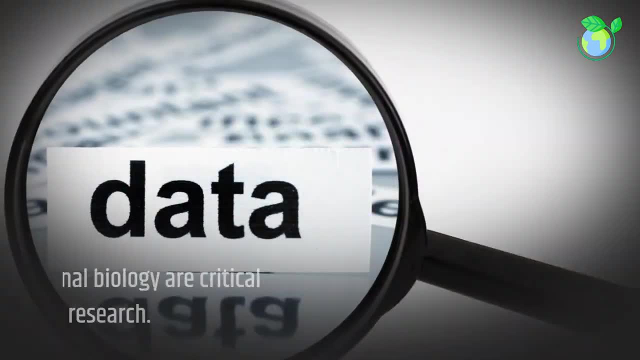 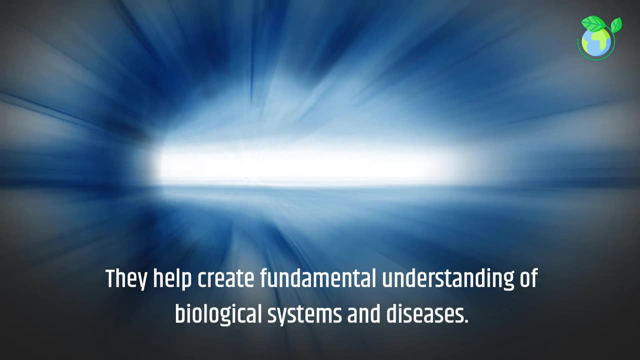 Computational biology helps researchers simulate and predict complex biological phenomena. They can then make inferences. They can then make informed decisions about future experiments. Bioinformatics and computational biology are critical tools in life science research. They help create fundamental understanding of biological systems and diseases. 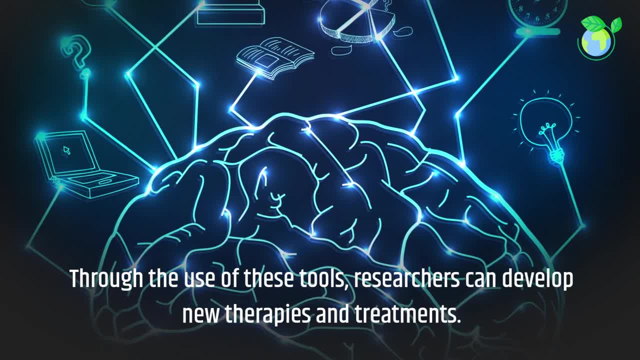 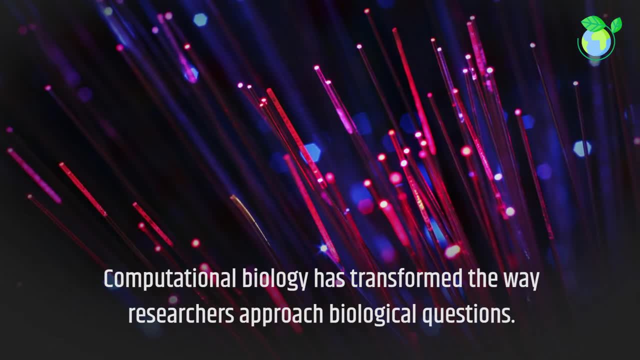 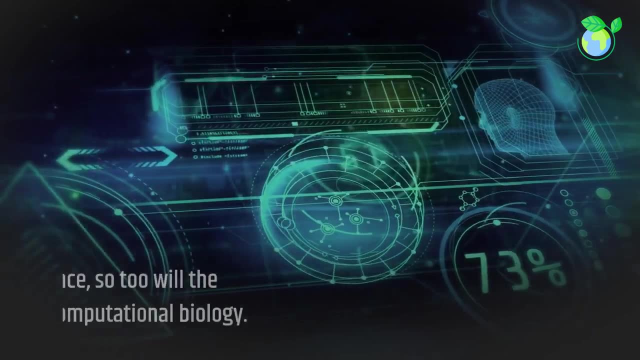 Through the use of these tools, researchers can develop new therapies and treatments. Computational biology has transformed the way researchers approach biological questions. It has enabled us to gain a deeper understanding of the complex biological systems. As technology continues to advance, so too will the applications of bioinformatics and computational biology. 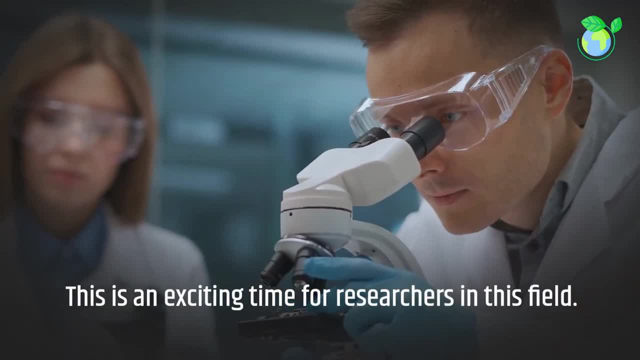 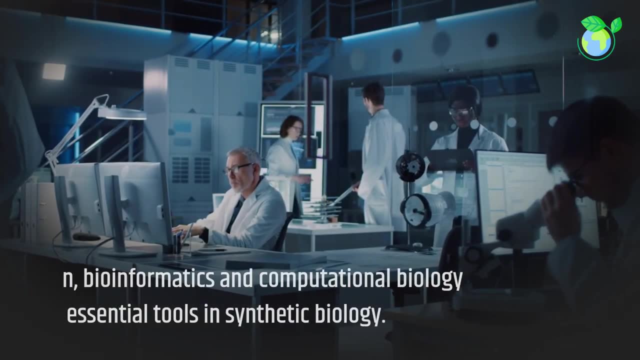 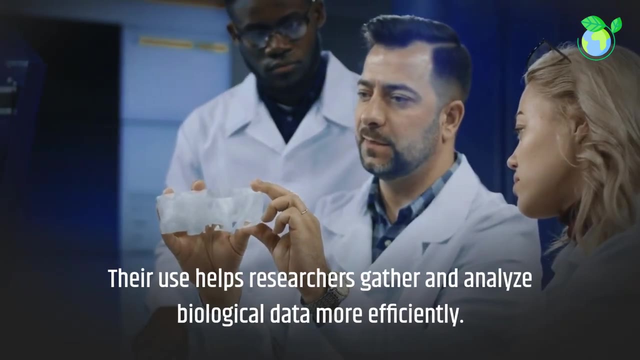 This is an exciting time for researchers in this field. Through the use of these tools, they will continue to unlock the mysteries of life. In conclusion, bioinformatics and computational biology are essential tools in synthetic biology. Their use helps researchers gather and analyze biological data more efficiently.